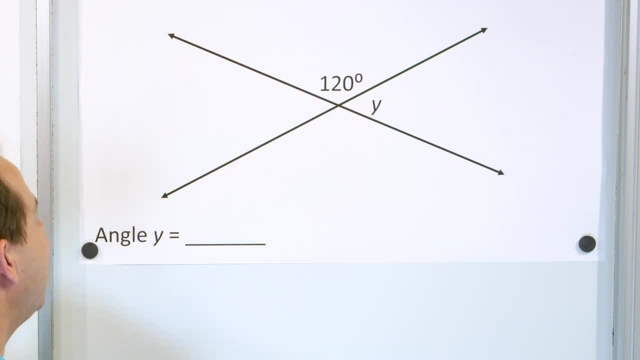 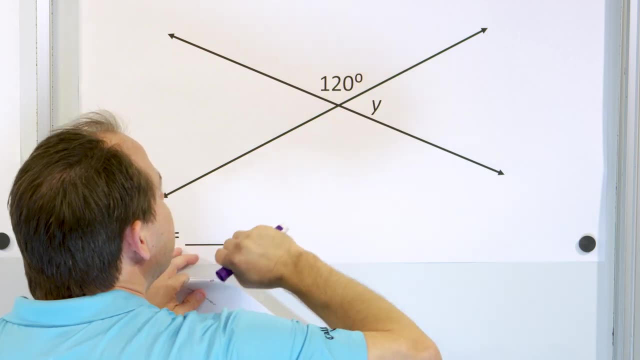 Except now we have angle Y over here and we're trying to figure out what is the angle Y? Now you need to start getting in the habit of seeing, when you see these straight lines that are broken up by another segment or a line. These are what we call supplementary to each other. They add up to. 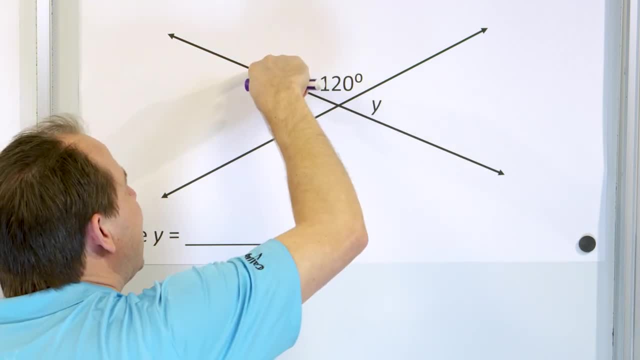 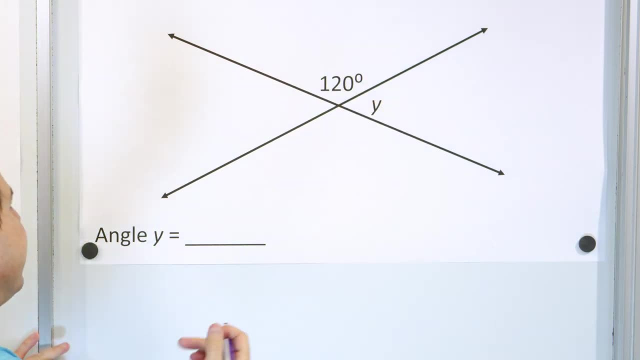 180 degrees. And you know this because any angle on a straight line from one side to the other has to be 180 degrees. So this plus this has to be 180. So in equation form, what you would say is 120 plus whatever Y is in degrees. 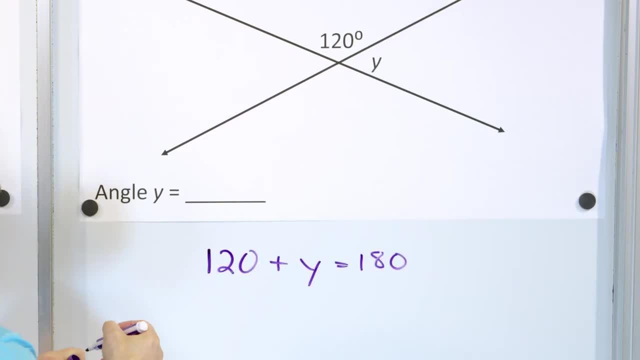 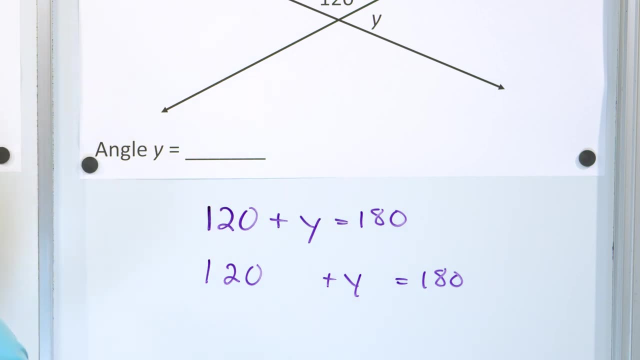 This is what it means to be supplementary. Now, in order to solve this, we'll just kind of spread it out a little bit and ask ourselves: how do we get Y by itself? Well, we have a positive 120.. So we'll subtract 120 from the left and subtract 120 from the right And on the left, of course. 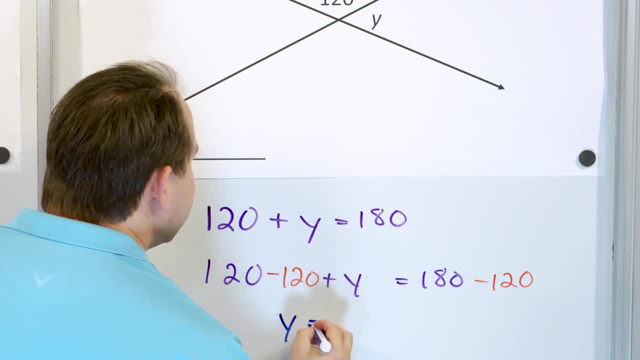 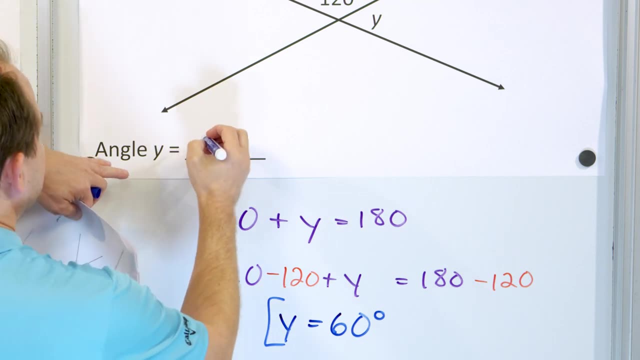 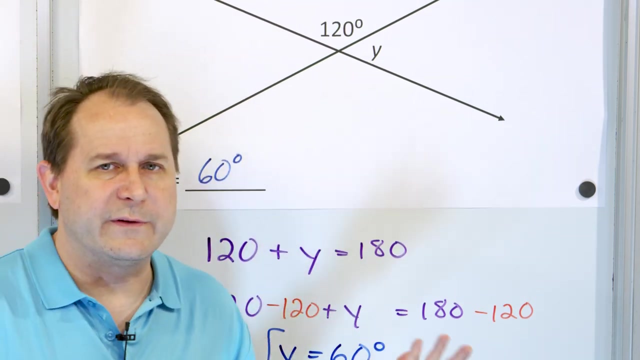 the 120 minus 120 is zero. So all we have left is Y, and 180 minus 20 is 60 degrees. So just put 60 and the unit is degrees. So this is what I was saying a minute ago. You can just solve these with subtraction. You know that. 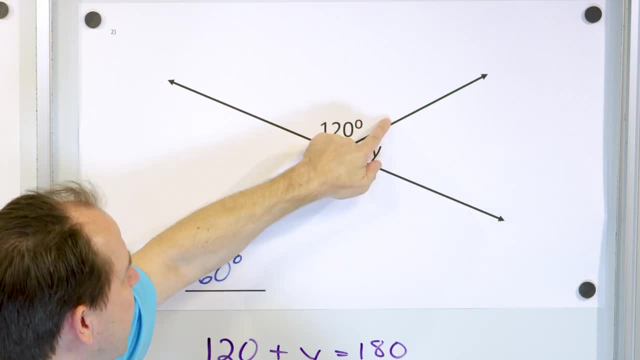 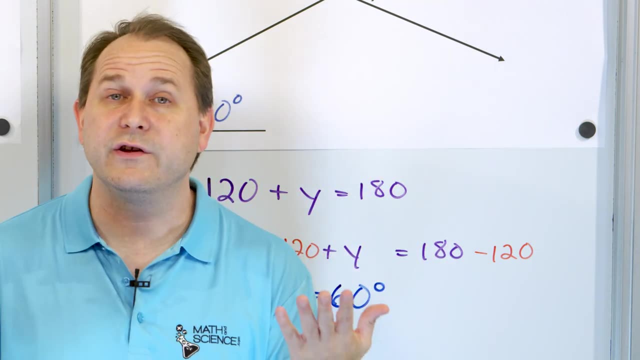 this has to be a large angle of 180.. Subtract this away Minus the 120 has to be what you have left. So you can do that, But I am writing them in terms of equations and subtracting from both sides, because I want you to get practice with this kind of procedure with equations. 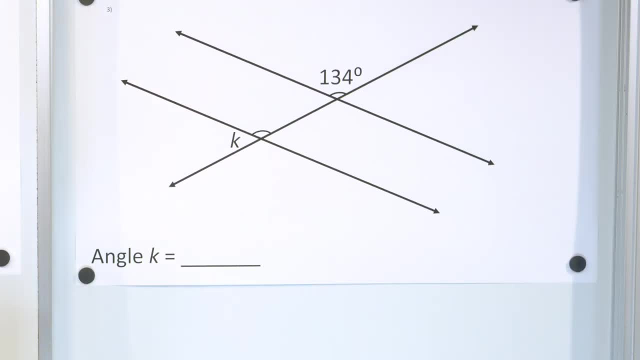 All right, So 60 degrees. That was the answer there. Let's take a look at problem number three. What is the measure of angle? Okay, Here Now. at first you're not really sure what to do, because K is way off by itself and you. 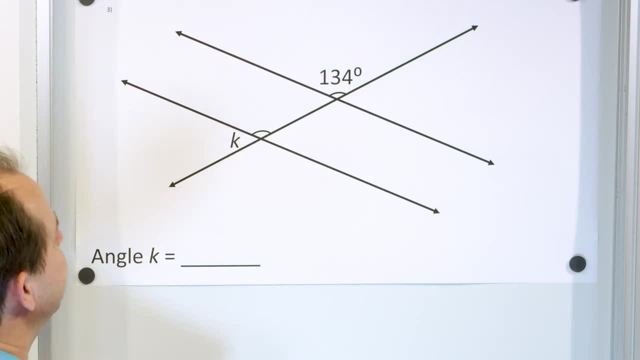 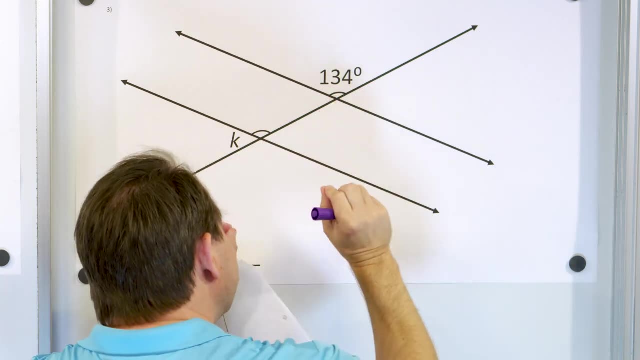 don't really know anything about what's going on over here, But you need to learn how to read geometric diagrams. When you see like an angle marking here and then there's like another angle marking there And if it's a true geometric diagram it's, like you know, congruency marks. 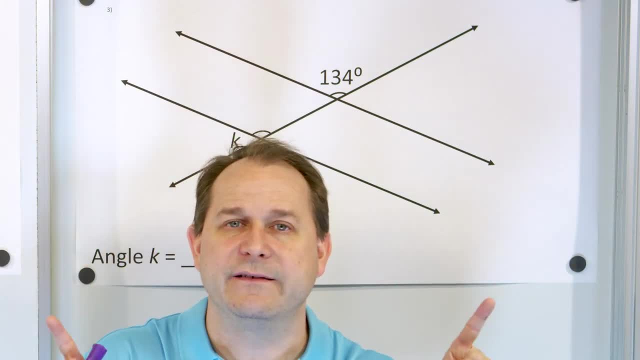 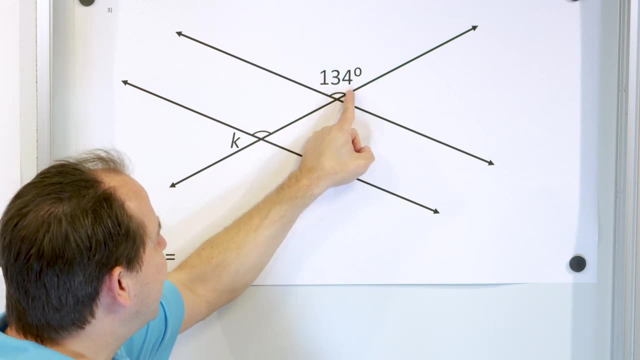 when you want to tell you, when you want to tell me that the length of the sides are the same, you put a little mark on the sides. Well, for angles, if you put a little mark here or a little angle arc, and it matches the length of the sides, you put a little mark on the sides And then you 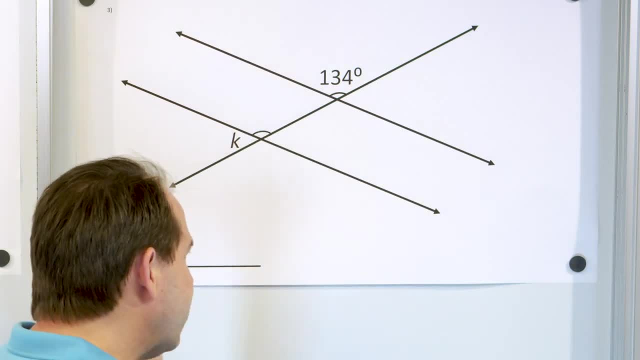 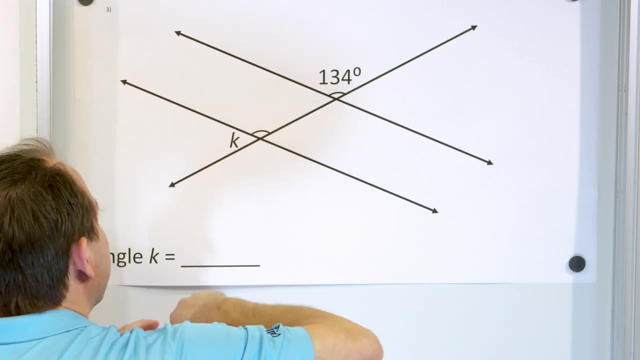 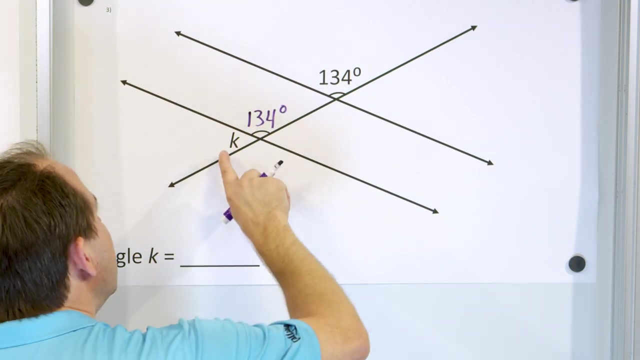 can assume those to be equal if it's a proper geometric drawing, right In this case. So what you know is that this is 134 degrees, but even though it's not written there, you know that this is also 134 degrees. So then, how do you find K? Well, this must be a total of 180.. So what you 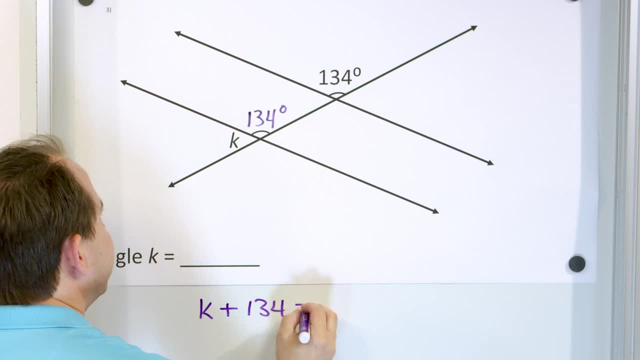 say: is K, whatever it is, plus 134 must equal 180, because this plus this must then be 180.. So then you just solve it: So K, whatever it is, plus 134 must equal 180, because this plus this must then be. 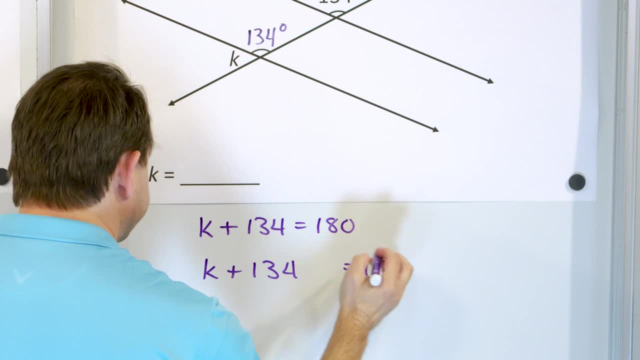 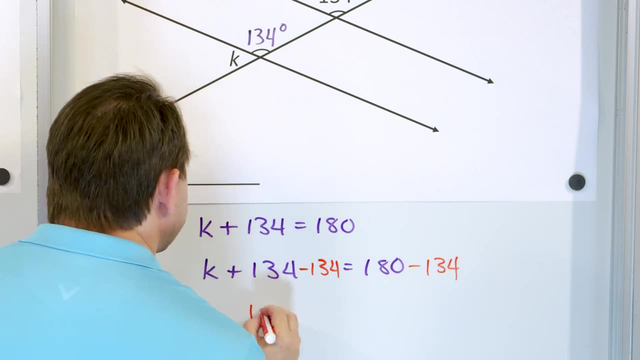 180 plus 134 equals 180. And then we'll just subtract 134,, subtract 134. And what we will get on the left is K. because this just disappears. K is going to be equal to 46 degrees Circle. that. 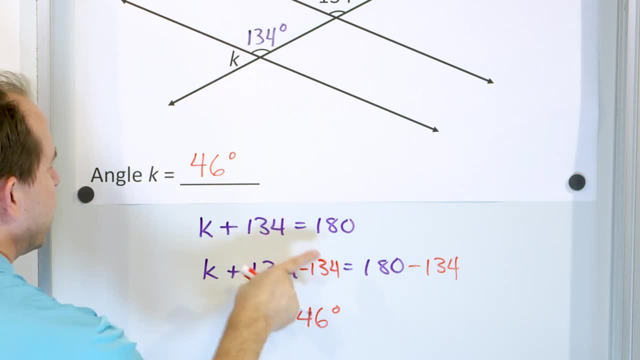 So 46 degrees, And you can check it by putting 46 back in here. The six and the four would bring it up to 140, and the 140 plus the additional 40 is 180.. So that is the correct answer. Let me take these down. We have a few more problems in this lesson. 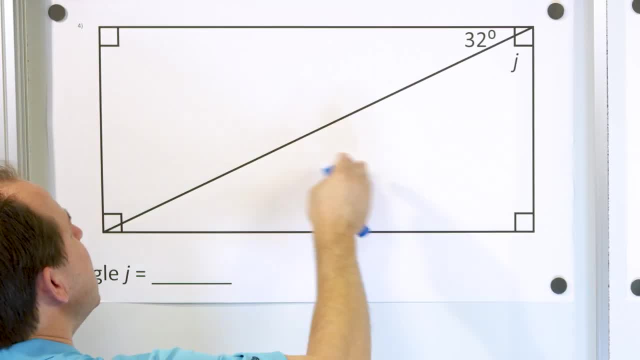 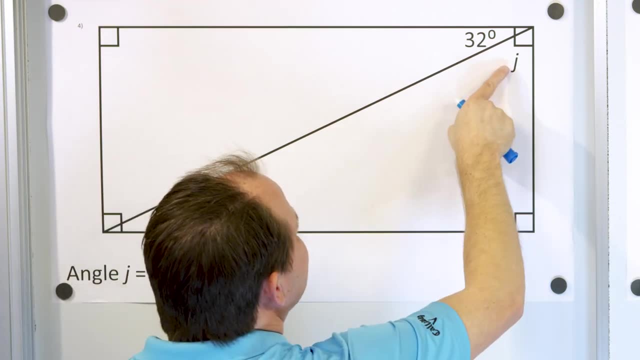 All right, here is problem number four. We have this kind of rectangle here, but we have a rectangle where corner to corner it is sliced in half here And we're trying to find angle J. So on the diagram, that is this angle measured from this segment here over to. 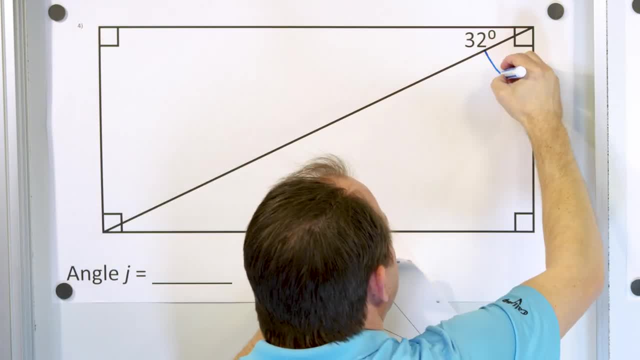 this one. So this is angle J. If you need to visualize it, you can kind of draw a little arc like that. That's angle J. Now what do we do? We know that these corners here, these little squares, indicate 90 degree angles. We know that these corners here, these little squares indicate 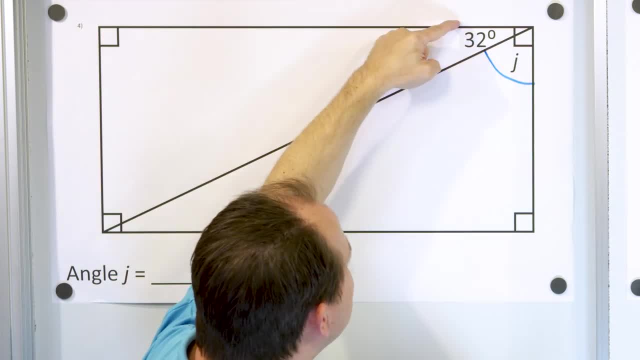 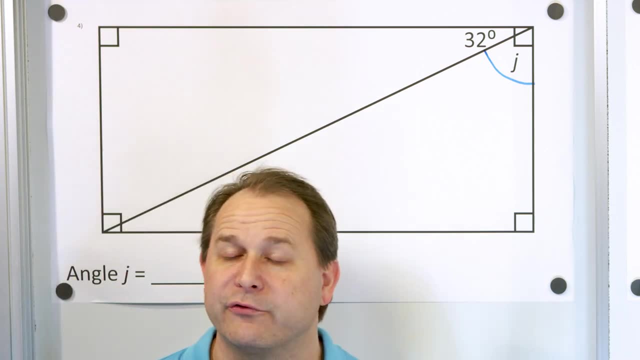 90 degree angles. We know that these corners here, these little squares, indicate 90 degree angles. So up here, what it means is 32 degrees plus whatever J happens to be must be equal to 90.. So these are complementary angles. Remember, supplementary means: they add to 180,. 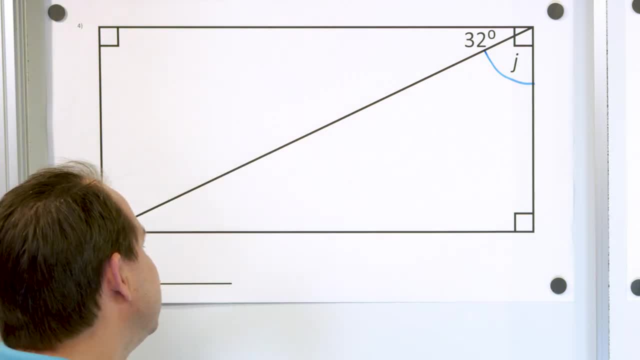 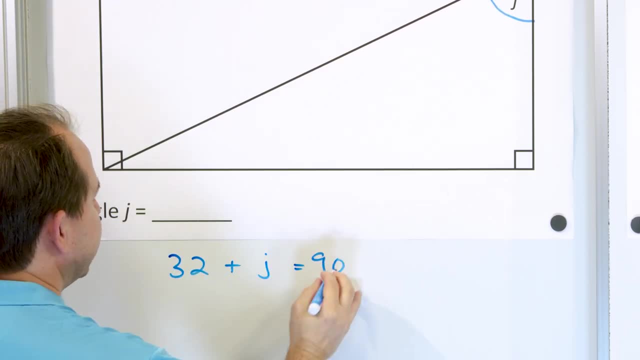 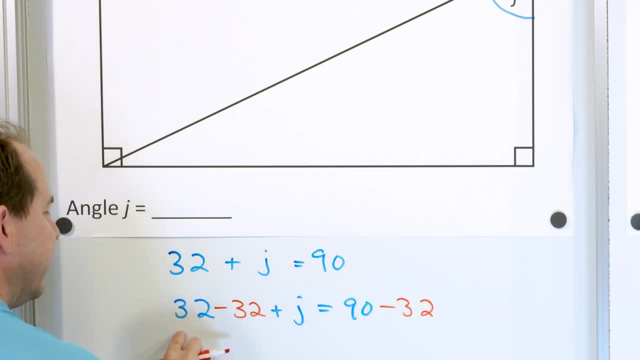 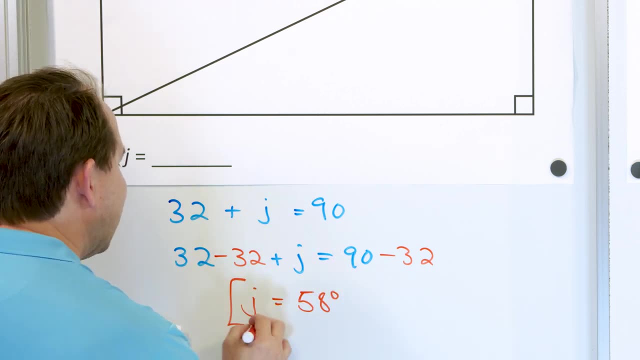 32 from the left, we'll subtract 32 from the right And this will be zero, So we'll just have J by itself. What is 90 minus 32?? That is 58 degrees, And you can check it by putting 58 back. 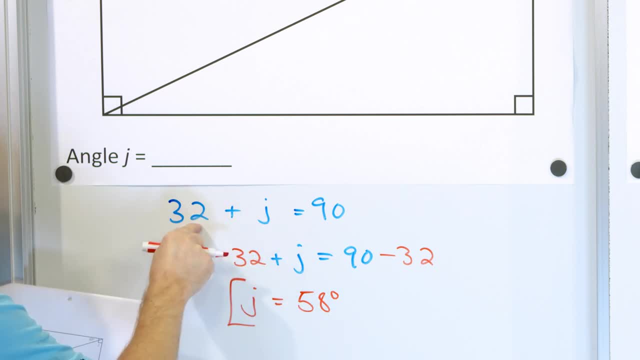 in here and adding it to 32.. If you add, put 58,, the two will make 60, and then 70,, 80,, 90. And so that makes sense. So the answer is 58 degrees for J, 58 degrees. All right, Let's take a look at. 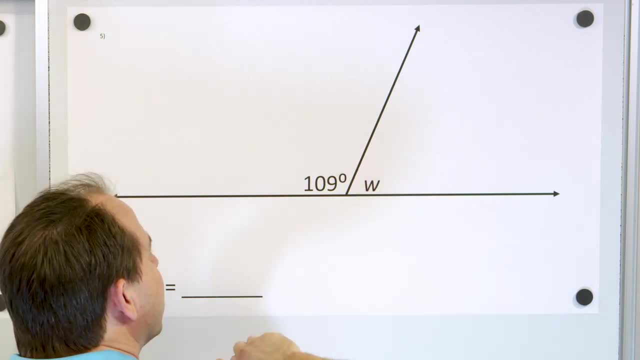 problem number five: What is the measure of angle W right? So this angle from this ray down here? Well, we know that this from this side of the line all the way to the other side must be 180.. So these are supplementary angles. They add to 180.. So 109,. 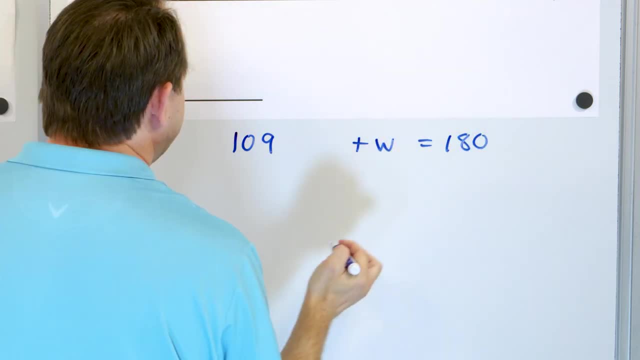 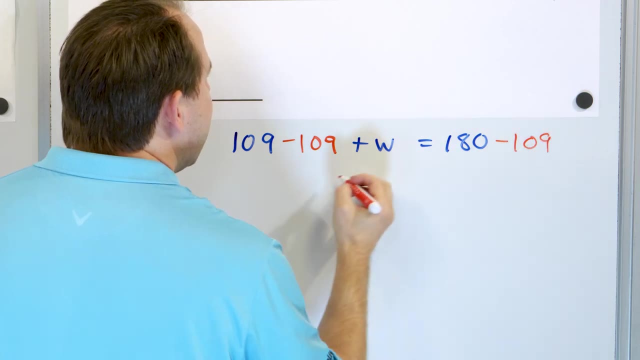 right, Plus whatever W is has to be the same as 180, right, But we want to get W by itself, So we subtract 109,, subtract 109. And the only thing you'll have left is a, because this goes to zero. 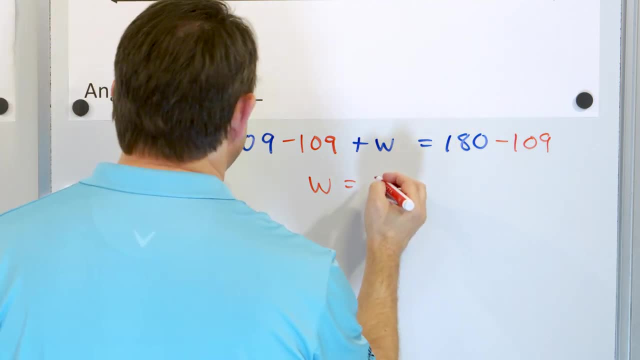 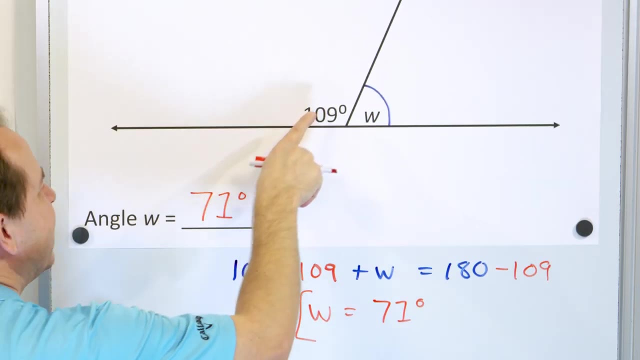 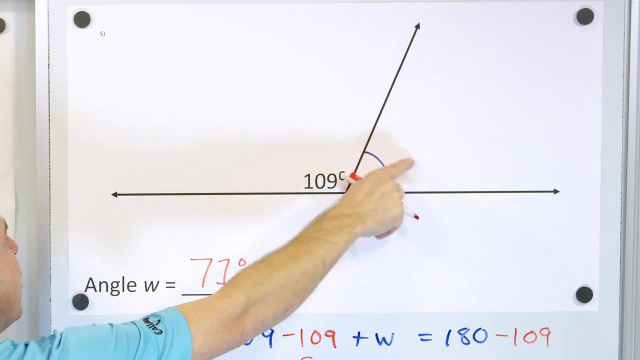 W. And then what is a 180 minus 109?? You get an answer of 70.. 71 degrees, So 71 degrees. Check yourself: If you put 71 in here and add to 109, the one will make 110, and then 70 more will make 180. And you know the whole thing has to be 180 degrees. This is 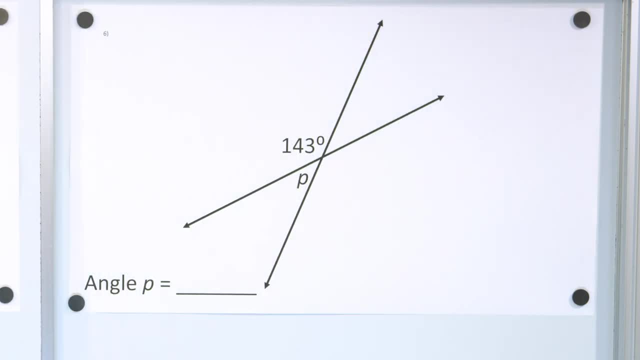 actually why we learned about complementary and supplementary angles? because it helps us solve problems, because we geometrically know it has to add to 180. And so we have. we define those terms for that reason. All right, Let's take a look at this problem. 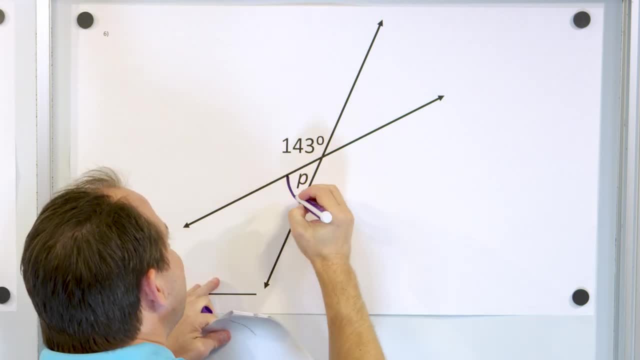 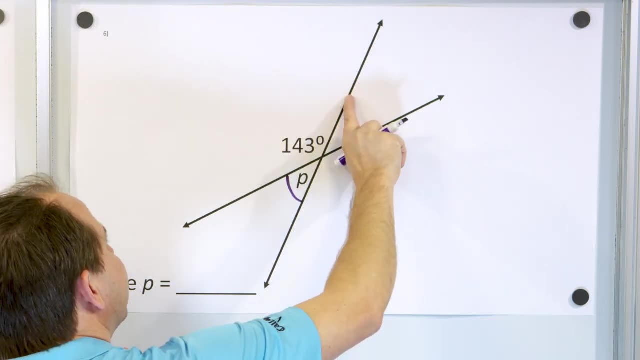 What is angle P? That is this angle right here between the rays. Now, maybe a little hard to see, you may have to turn your head sideways, but this is a line and the angle that goes from this side all the way to the other side again has to be 180.. So when you add this angle plus this angle, 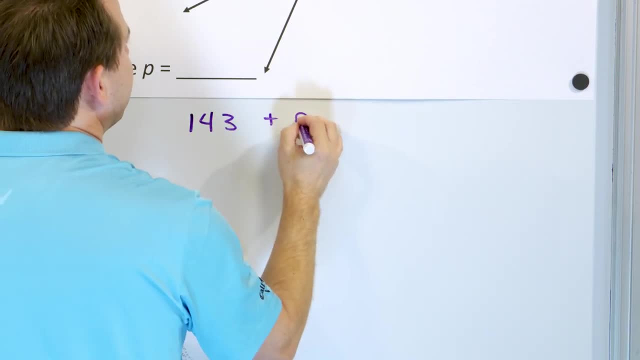 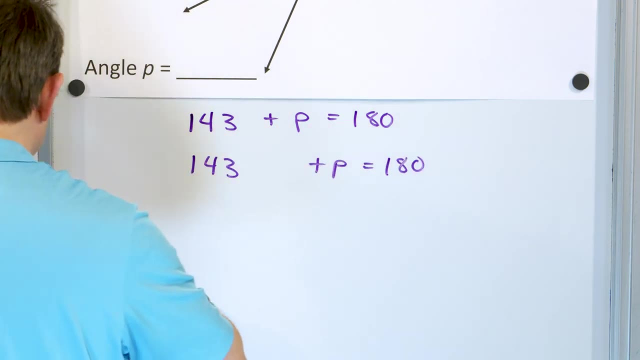 it must be 180.. 143 plus whatever P is has to be 180.. So 143, just spread it out, So I have a little room. How do I get P by itself? I'm just going to subtract 143.. 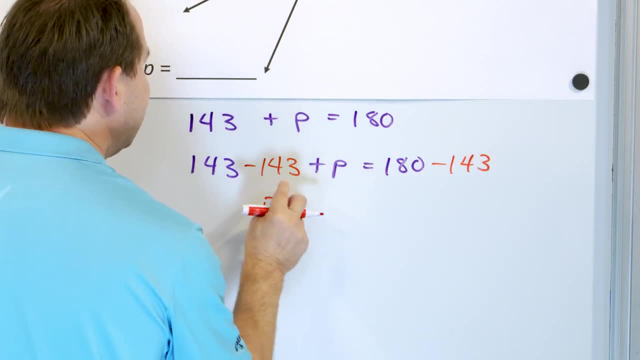 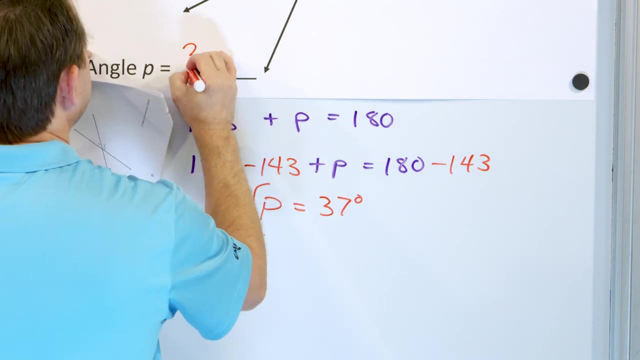 Subtract 143.. All I have left on the left is P, because this goes to zero. And what is 180 minus 143? 37 degrees. So 37 degrees. You can check it by putting it back in here, The 7 going in here. 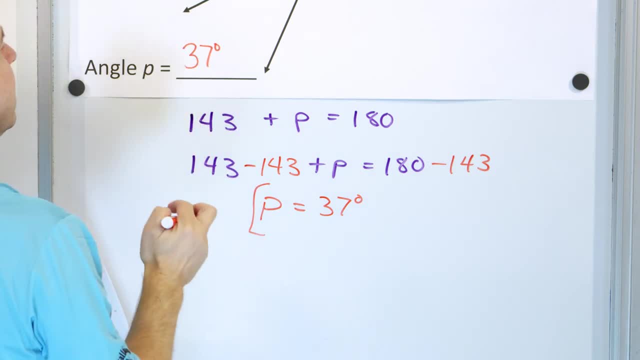 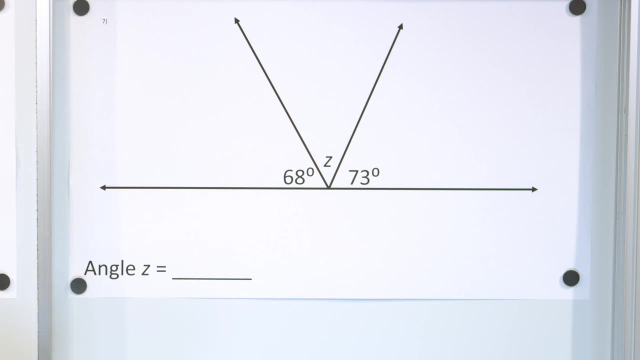 will make 150, and then 160, 70,, 80, with 30 more, And that's the final answer. All right, Here is number seven. Now, this is where it starts to get a little more useful to write things as an equation. 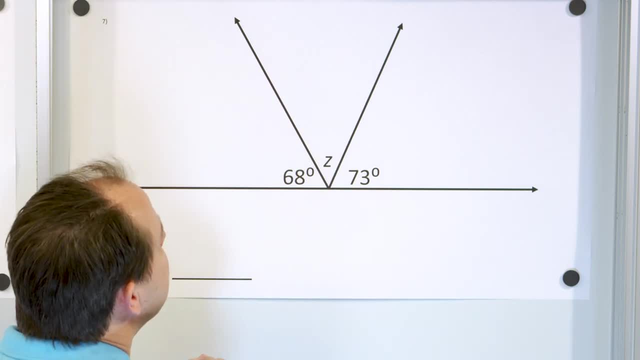 because you're going to have to do a lot of things. You're going to have to do a lot of things. You're trying to find angle Z, but this looks like a totally different situation than what we have covered before. We have lots of situations where we've had just a line and it's cut in one place. 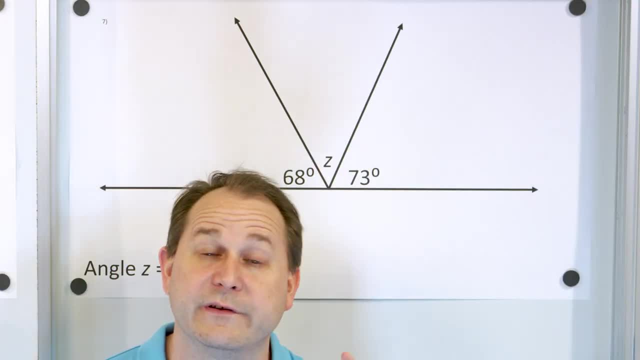 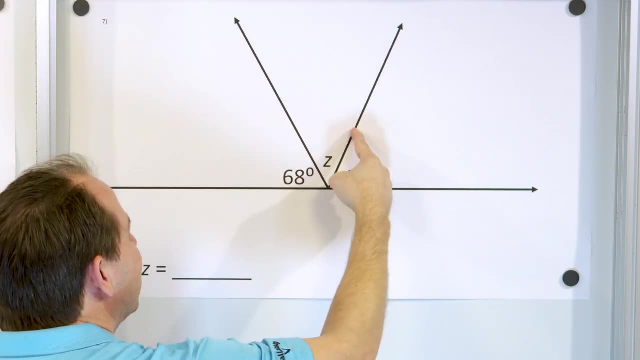 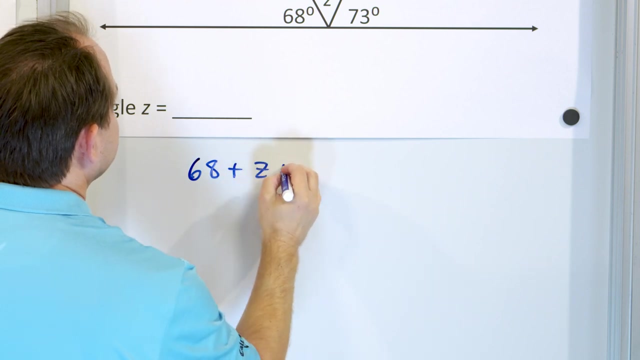 and we know they add to 180.. So at first you look at this and you're not totally sure what to do, until you realize that this must all be 180 degrees. So this angle plus Z, whatever it is, plus 73, all of them together must equal 180. So 68 plus whatever Z is, plus 73 must all together. 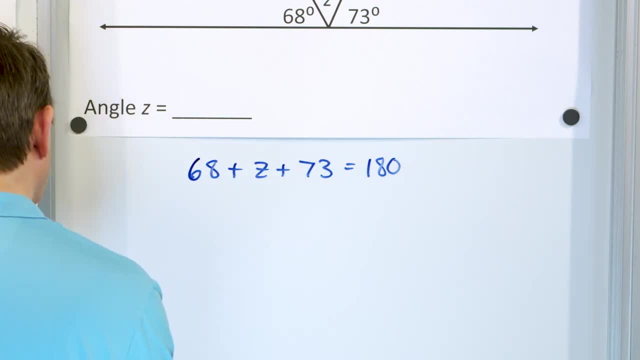 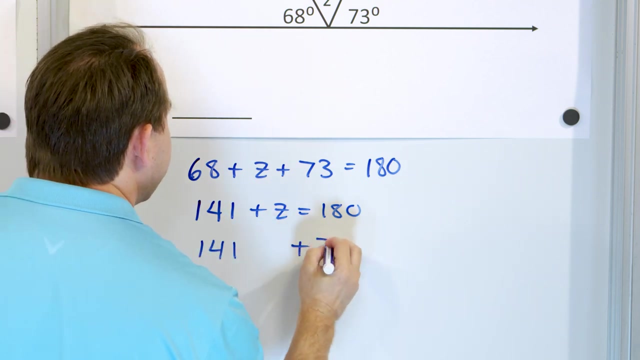 add up to 180 degrees, All right. Now, when you add 68 and 73 together, you're going to get 141. Right? So how do we solve for Z? Just spread it out And I can do what I want to both sides. So. 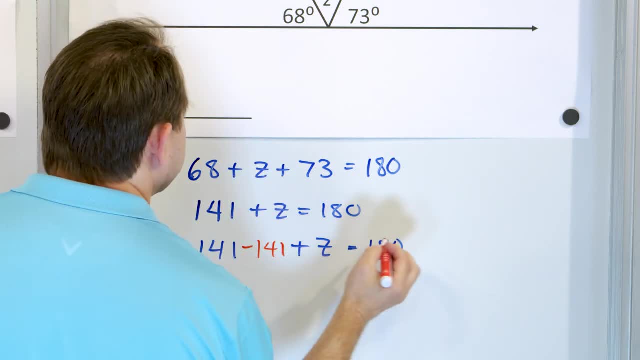 I'm going to subtract 141.. 141 from the left, 141 from the right, So it disappears here. So Z is going to be equal to 180 degrees. So I'm going to subtract 141 from the left, 141 from the right. 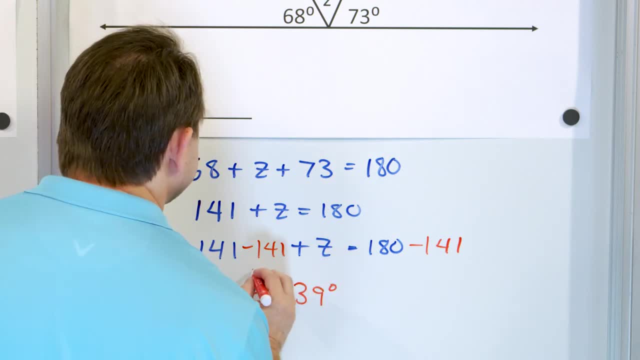 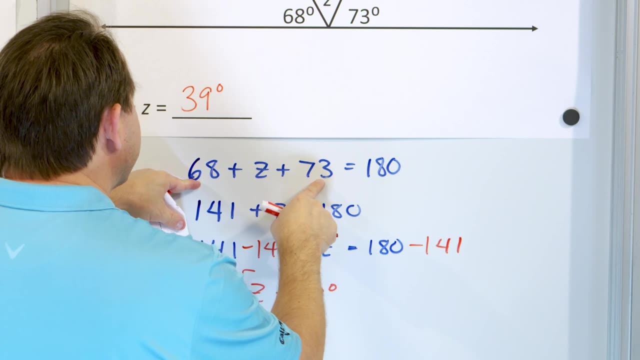 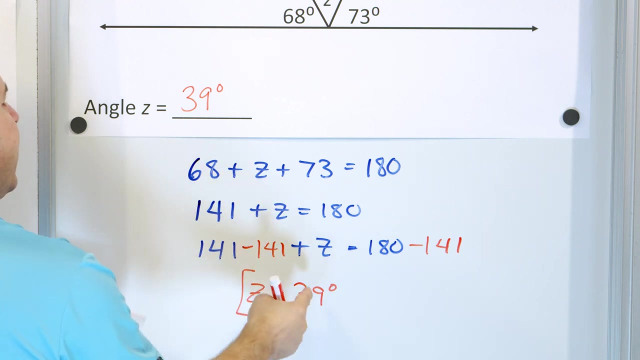 Z minus 141, 39 degrees. So 39 degrees And you can check yourself, because we just figured out that these two together, when we add them together, comes out to 141. So if you put 39 in there and add it to this, it'll be the nine, will go in and make 150 and then 160,, 70,, 80,, 180 when. 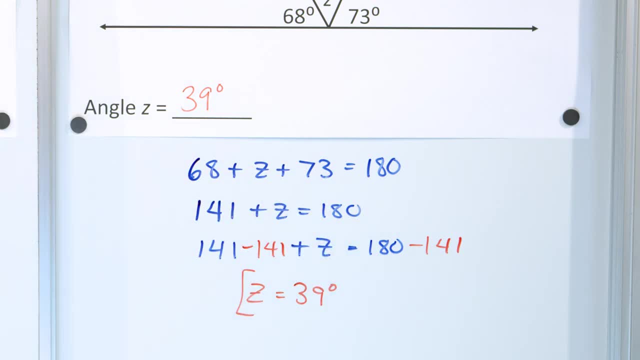 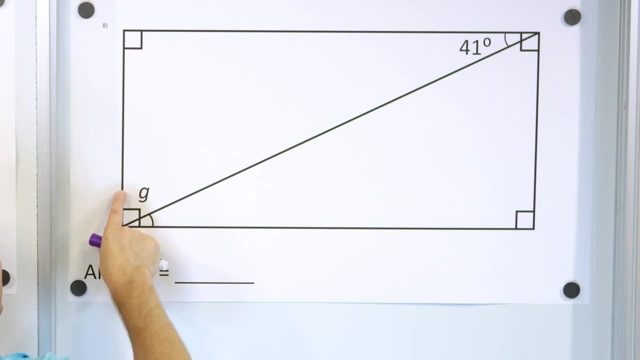 you add that 30 more, So it's 39 degrees. Let me take this one down. We have one more and call it a day. Okay, Here's our very last problem. We're asked to find the measure of angle G, but it looks a little weird because on this side over here we don't really have any other. 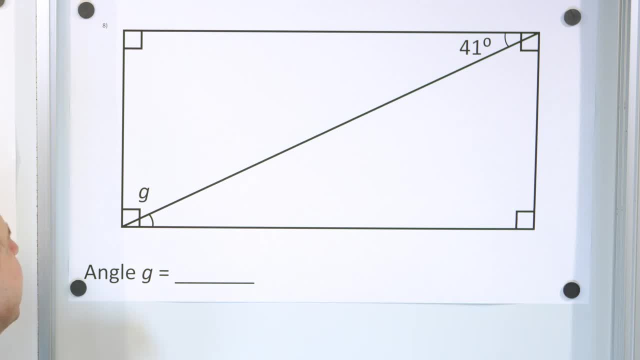 numbers. But what we have figured out is that there's a couple of different ways to tackle this, right? First of all, you notice that this is 90 degrees, right? So the whole thing is 90 degrees because of the square right here. So we could find G if we only knew what this angle was. 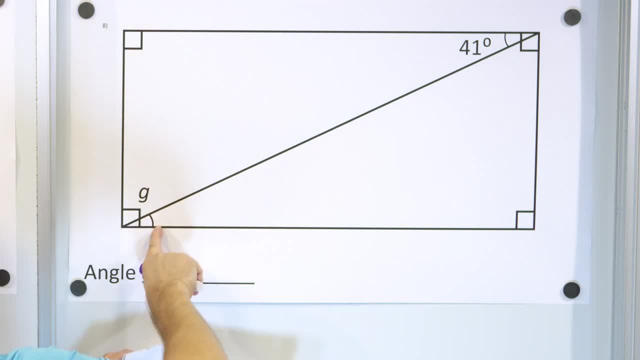 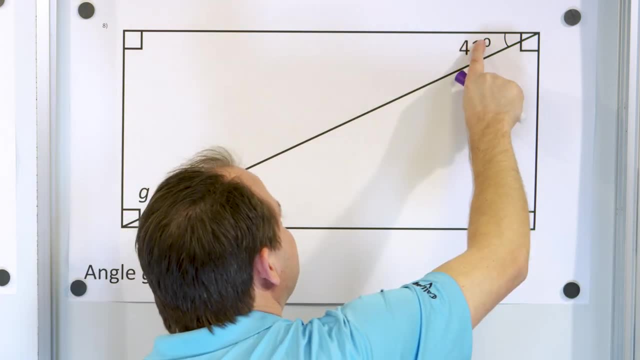 but it's not really written here. But then we realized- wait a minute, it has an angle marking and over here has another angle marking. So because this angle marking matches this one, we know that this, this angle, is the same as this angle. In fact, it looks to be about the same, doesn't it? So 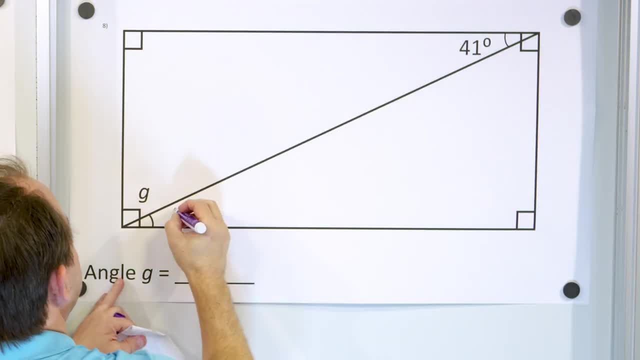 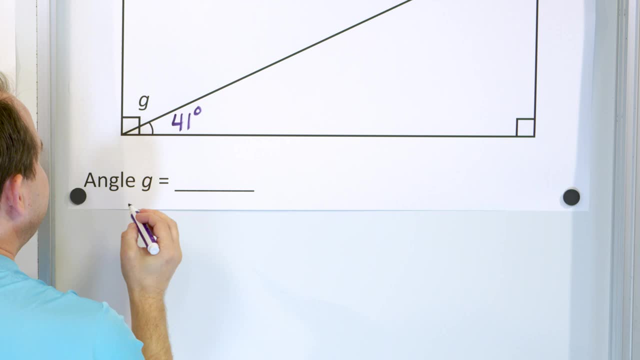 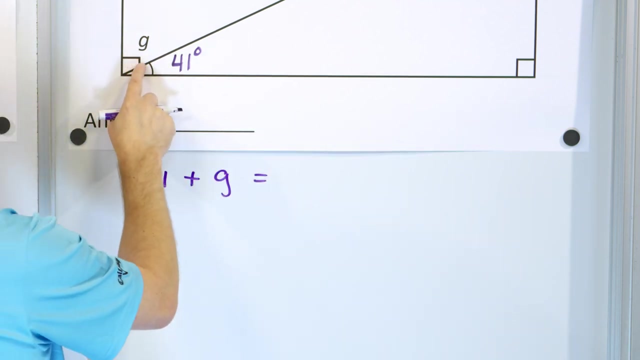 actually this 41 degrees is the same as this one down here, 41 degrees, And you know that because of the angle marking here, right Now that you know that this is 141 degrees, you can write down that 41 degrees plus whatever G is has to equal what? 90, because this is a 90 degree angle. 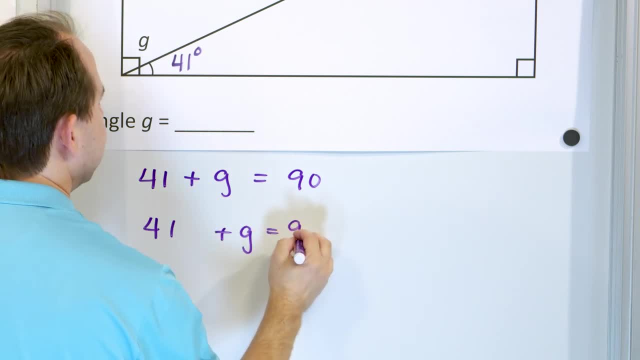 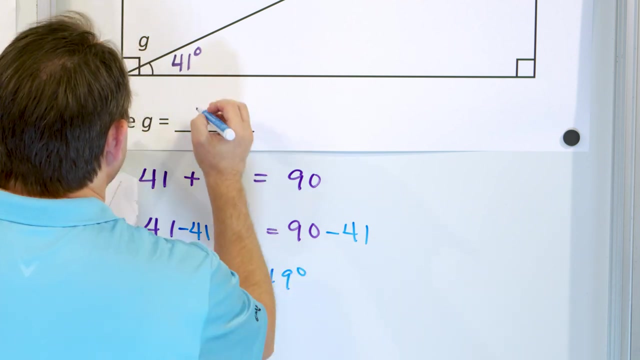 So we'll just solve that equation. How do we do it? Well, let's just subtract 41. This gives you zero. So all you have is G, 90 minus 41 comes out to be 49 degrees. 49 degrees- And double check yourself. You put 49 in here and you add one more. that'll. 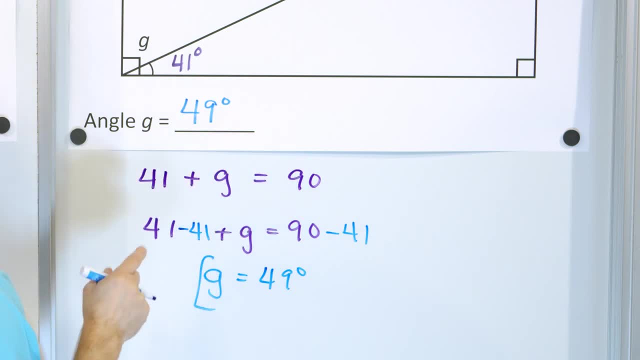 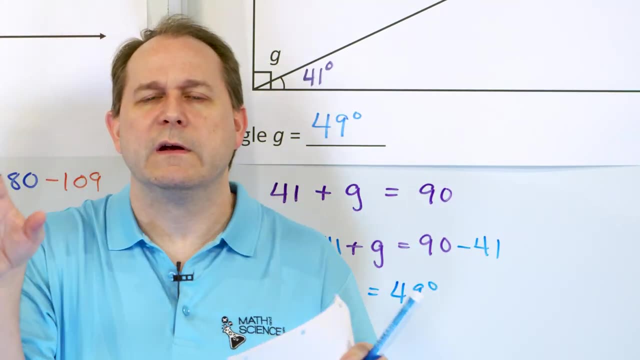 be 50. And then the 50 plus the 40, leftover is the 90. And so you've verified that it is 49 degrees. So this lesson was kind of you know, it's kind of an all around measuring angle. 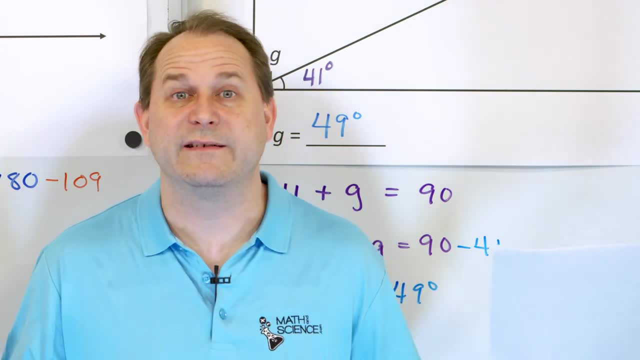 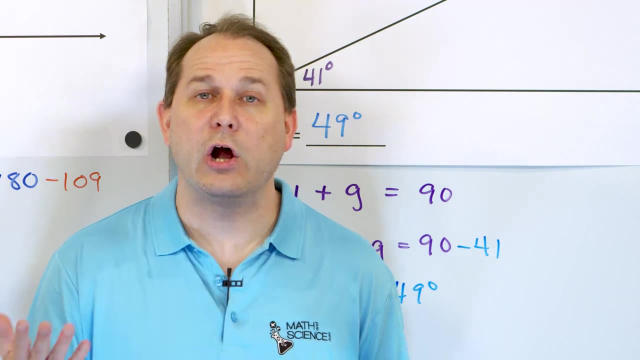 calculating angle kind of lesson. You know, it's kind of a hodgepodge of lots of different things. Basically, what we have is situations where draw figures and ask you to calculate the angle And, as I said at the beginning, you can solve all of these by addition and subtraction If you look. 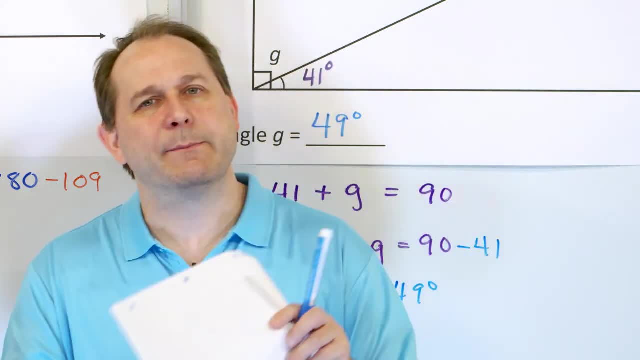 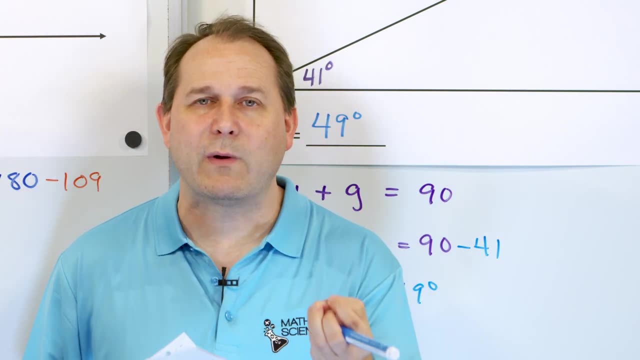 back through all of them. they're all solved by taking 180 minus or 90 minus and you can do it that way. But I like to write the equations down, especially now that we've done it so much, so that you can practice writing equations down, Because this kind of thing you'll be surprised when we 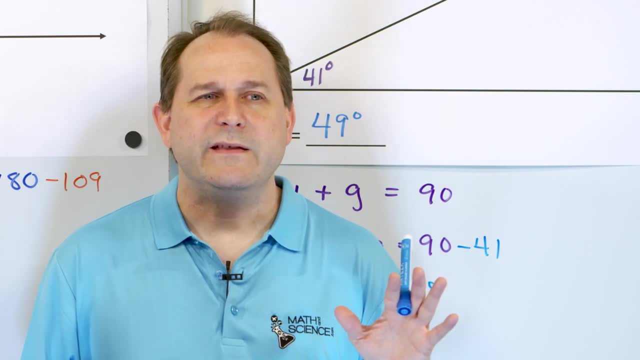 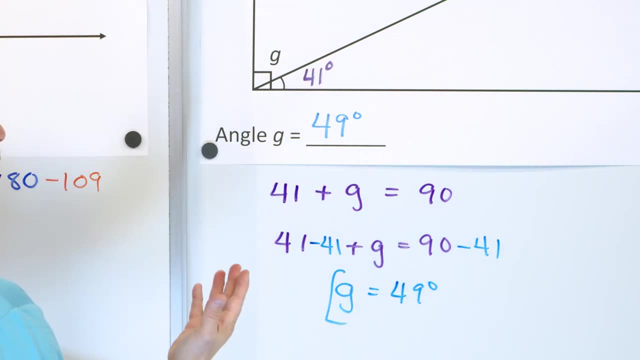 get into classes down the road in physics, where you're going to have to write the equations down, where the problem is easy to solve, but the student can't get there because they don't know how to write an equation now. So we have to start with simple situations where you know this plus.